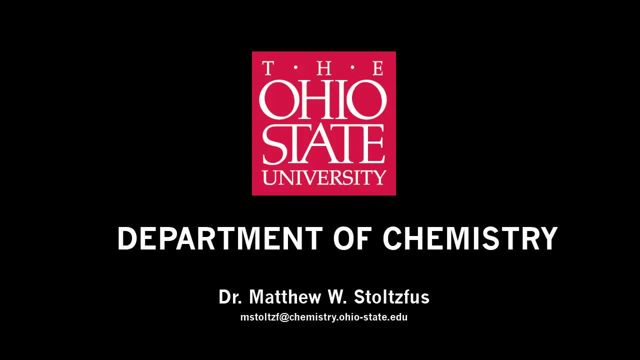 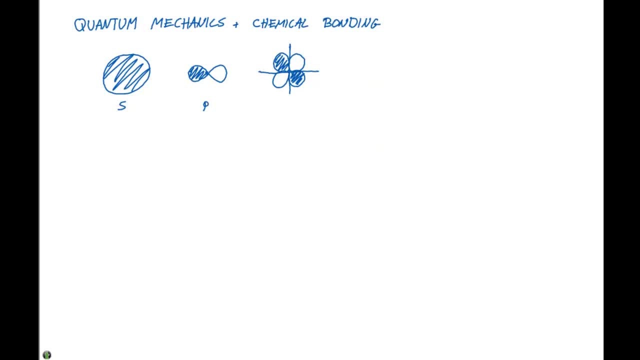 In this video we're going to talk about how quantum mechanics and chemical bonding are related, And this is going to eventually lead us to something called molecular orbital theory. So if we look at an, s, a p and a d orbital and their three-dimensional representations, 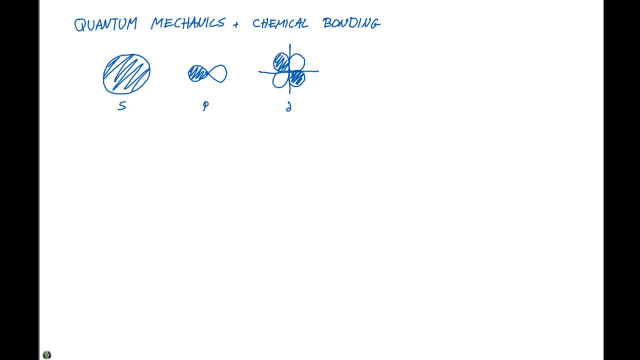 sometimes we'll shade each of these orbitals And the question is: why do we shade these orbitals the way that we do And what do the shapes really relate to? So the shape of an atomic orbital which are shown above corresponds to the probability. 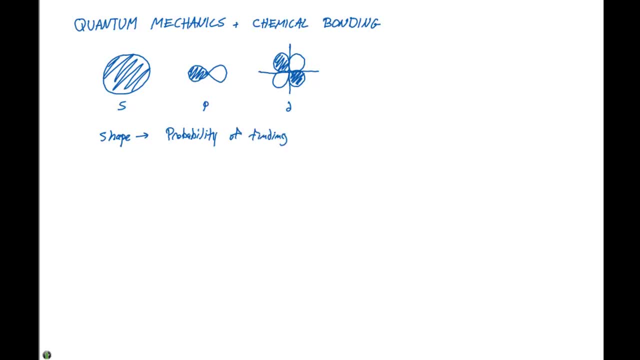 of finding the electron in a certain location, And sometimes chemists refer to these as probability density functions. So where is this electron in this particular orbital most likely to be found? Okay, Heisenberg has his uncertainty principle And he talked about how we don't know the exact location and 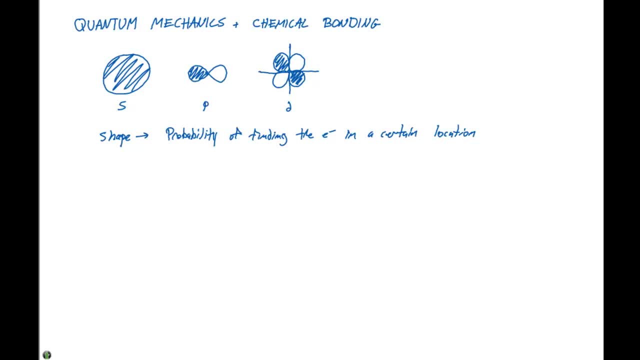 momentum of a particular electron. And this is because our electrons act as waves and particles, So we have to keep both of these in mind, And Schrodinger came up with an equation that said h psi is equal to e psi, And this psi part right here is called a wave. 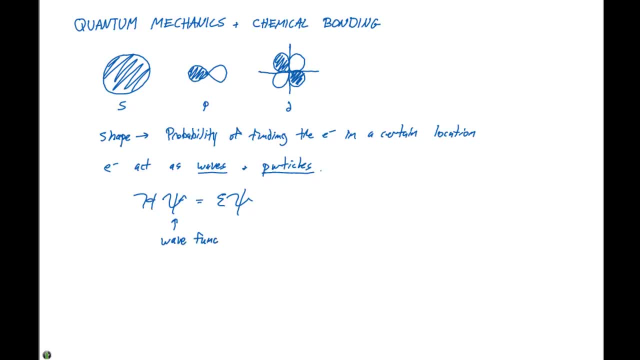 And this one right here is called a wave function, And this wave function is gonna describe the path of the electron, And we can relate this to differential mathematics. When we solve this equation, there's something called a node, And a node is an intermediate for a path. 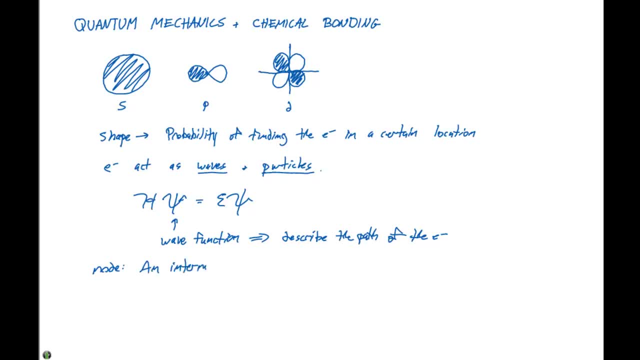 And a wavelength is a path, So the path of the electron. when you get to the path, or the path of the electron, it's like a sequence, An intermediate point at which the probability function goes to zero, So there's a zero probability of finding that electron at a particular node. 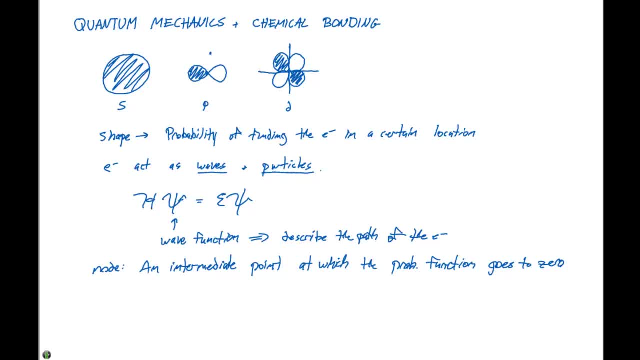 And if we look back up to the p and the d orbitals, the nodal plane for the p orbital is right here And the d orbitals for this particular d orbital are gonna lie right along the axis. okay, So when we look at nodes, 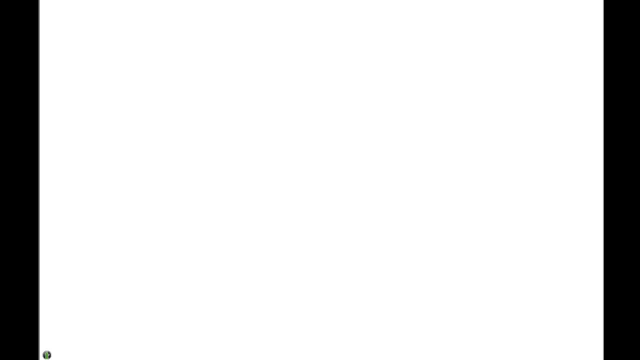 there are two types of nodes that we have to look at, And those nodes are radial and angular, And we can look at the various probability density functions to determine our radial nodes. So if we look at the radial nodes of an s orbital, We can get something like this: 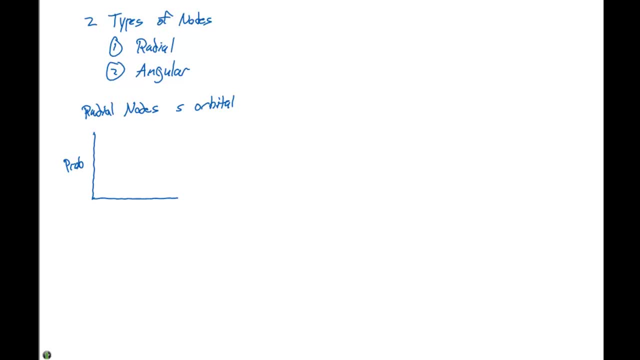 Where, if we put the probability of finding the electron on the y axis and the distance from the nucleus on the x axis for a 1s orbital, that probability function is gonna look something like this: Okay, where there's a main probability of finding that electron. 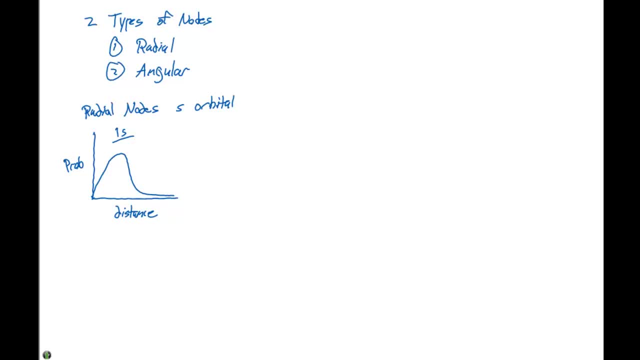 fairly close to the nucleus And there are no nodes here For a 2s orbital. if we plot the probability versus the distance, we're gonna see a graph that looks something like this: And at this point, right here, we have a node. 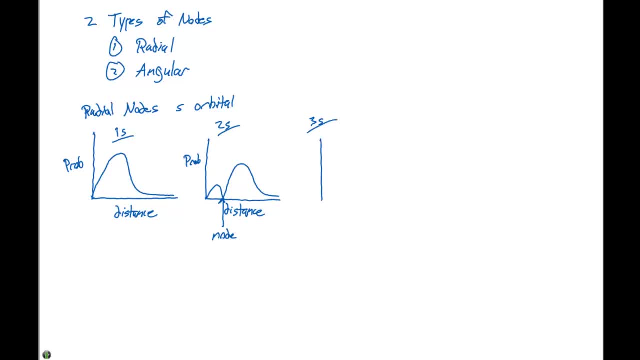 For a 3s orbital, if we plot the probability versus the distance, we're gonna find that there's two nodes there And the probability of finding that electron farther from the nucleus is gonna increase as we increase n, or the principal quantum number. 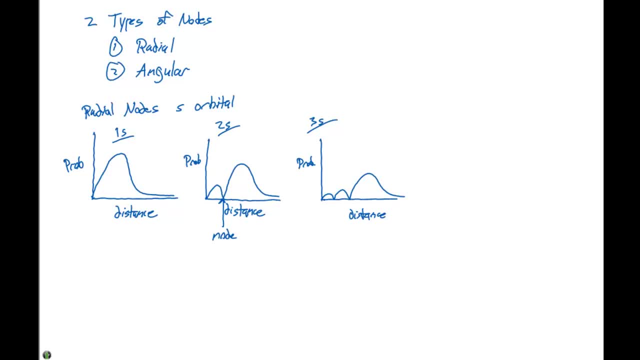 We also have angular nodes And actually, if we wanted to look at a picture of this before we get on to that, if we have our various s orbitals, the 1s, the 2s and the 3s- 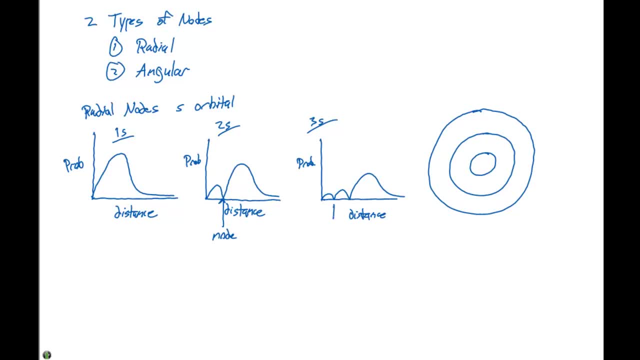 These two radial nodes will correspond to these lines right here in the 3s orbital. So the 3s orbital, if we represent it over here on the right, we'll have two radial nodes. Another type of node is called an angular node. 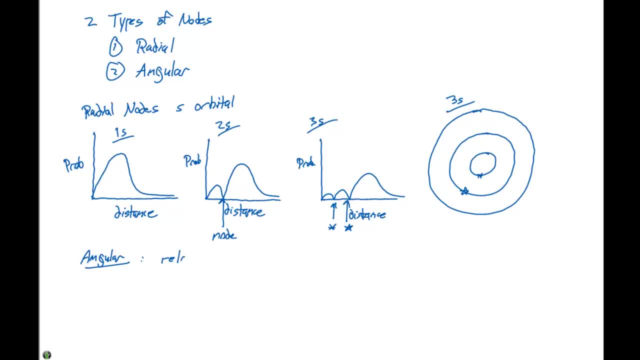 And the angular node is related to the azimuthal quantum number, which we abbreviate with an L, And we say that the azimuthal quantum number is equal to the radial number and that the radial number is equal to greater than 0.1. 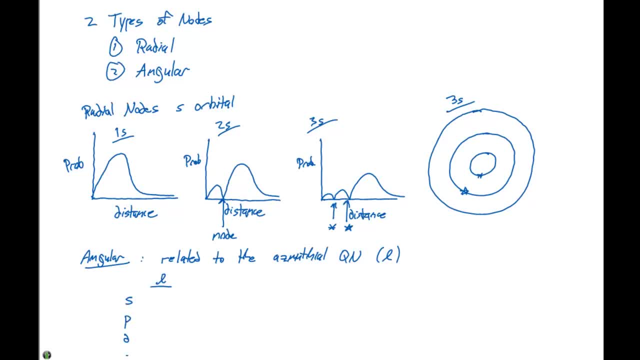 number L for S, P, D and F orbitals is 0,, 1,, 2, and 3, respectively. If we have an S orbital, it's completely spherical. There are zero angular nodes. For a P orbital, We have one angular node. 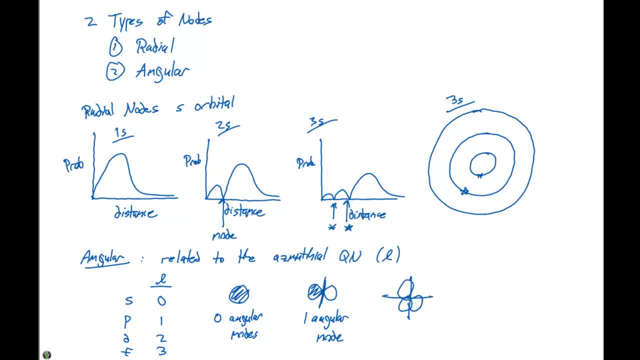 And for a D orbital, there are two angular nodes, And the number of angular nodes is gonna be corresponding to the L quantum number or the azimuthal quantum number. Okay, And all of these properties are related to the fact that the electron can act as a wave. Okay.